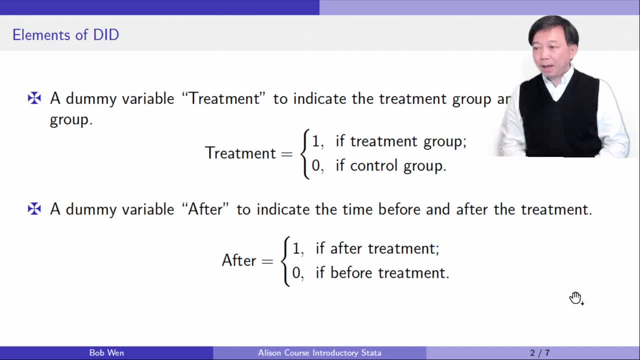 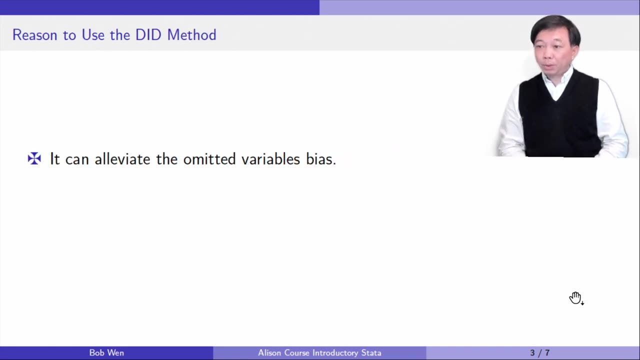 To figure out the treatment effect, we compare the outcomes such as health, wage or employment rate between the treatment group and the control group before and after the treatment. Why do we employ the difference-in-differences method? Because it can alleviate the omitted variable bias. 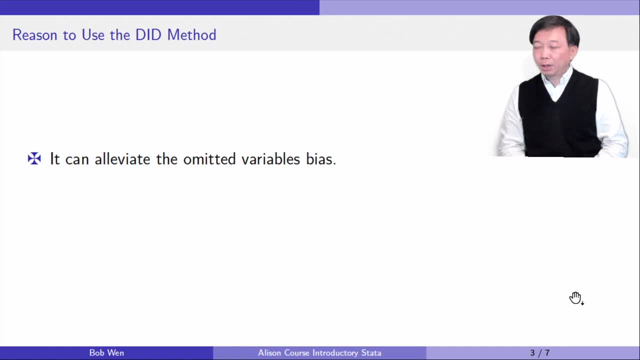 Suppose there were unobserved factors that influence the outcome variable. We could not include the unobserved or unmeasured factors in the model and therefore it could result in omitted variable bias. After difference-in-differences, the unobserved factors will be cancelled out of the model. 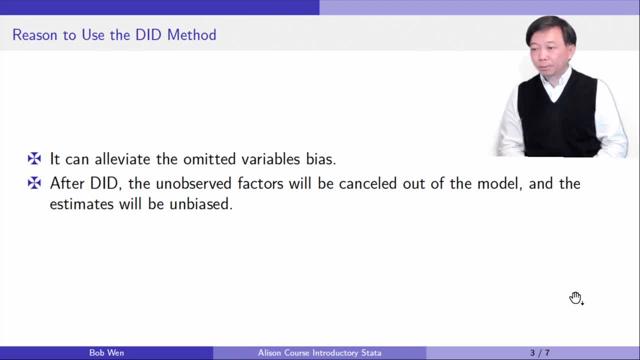 and the estimates will be unbiased. In other words, the estimate is the pure treatment effect which can better explain whether the treatment works and makes a difference. Let's see how we can do the difference-in-differences in the OLS regression model. 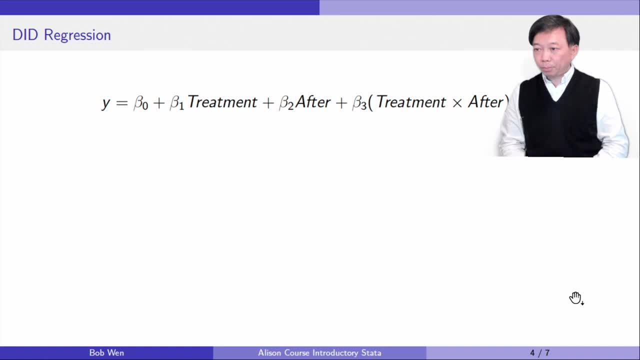 We include the interaction term between the treatment and the after variables in the model. The coefficient β3 on the interaction term measures the average treatment effect. For the control group, the difference between after and before the treatment equals β2.. For the treatment group, the difference between after and before the treatment equals β2 plus β3.. 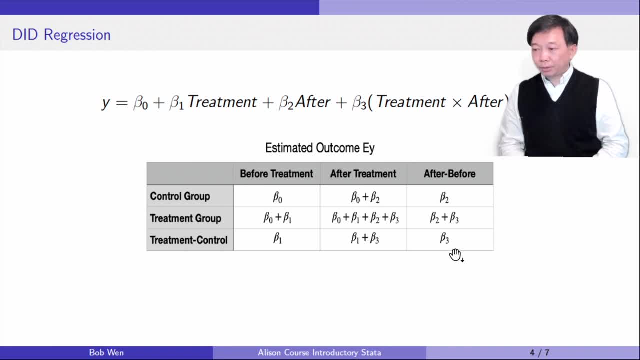 The difference-in-differences is β3.. β3 measures the pure effect of the treatment on the outcome, by ruling out other influences experienced by both groups. For instance, both groups of people may experience an economic downturn that is unobserved or unmeasured. 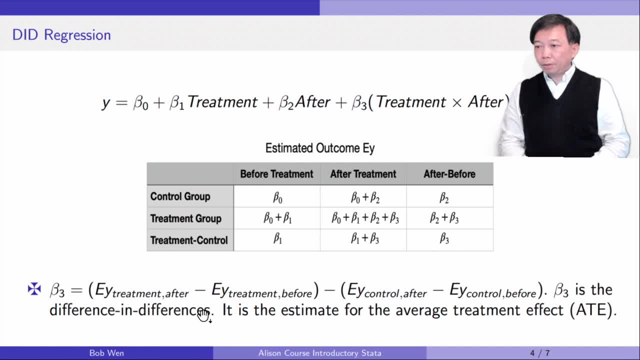 It is not captured by the model. Using the difference-in-differences method, we can account for these unobserved influences as if they were included in the model. It is important because these unobserved factors may lead to omitted variable bias if they are left out of the model. 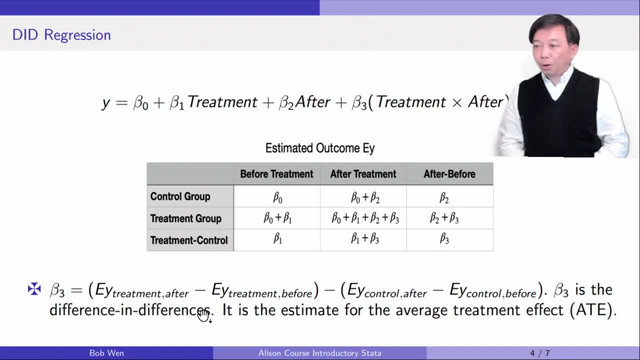 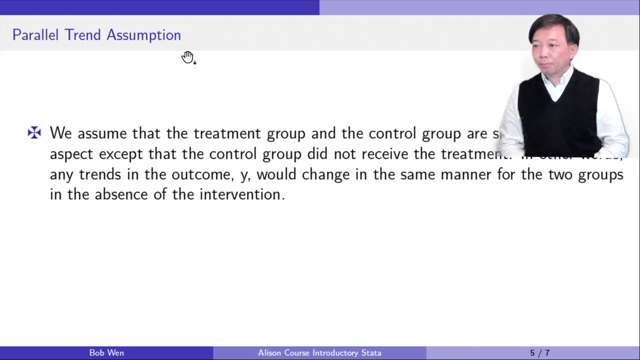 A crucial assumption for unbiased difference-in-differences estimates is the parallel trend assumption. We assume that the treatment group and the control group are similar in every aspect, except that the treatment group did not receive the treatment. In other words, any trends in the outcome y. 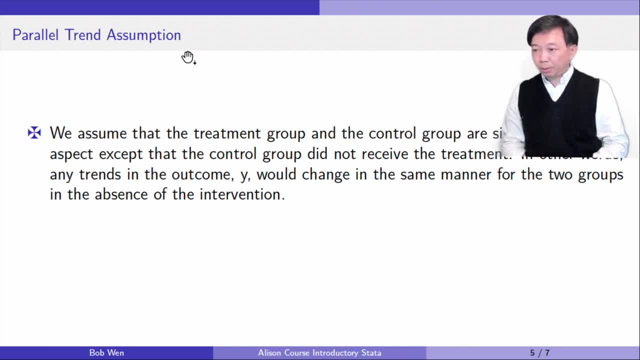 would change in the same manner for the two groups of people in the absence of the treatment? It is equivalent to saying that the unobserved factors impact the outcome variable in the same way between the control group and the treatment group. What if the assumption is violated? 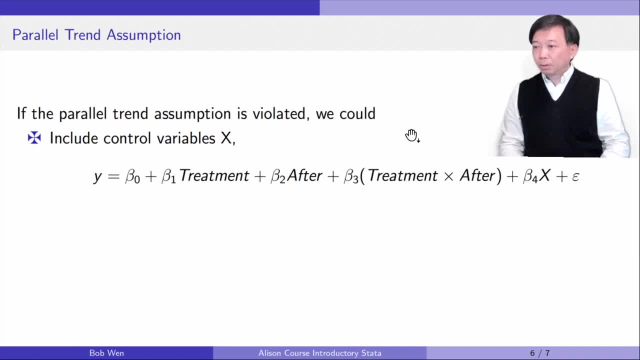 That is, the two groups are not similar. One solution is to include other observable explanatory variables as controls in the model. In this framework, the control variables account for the differences in the observable characteristics between the two groups that are not due to the treatment. 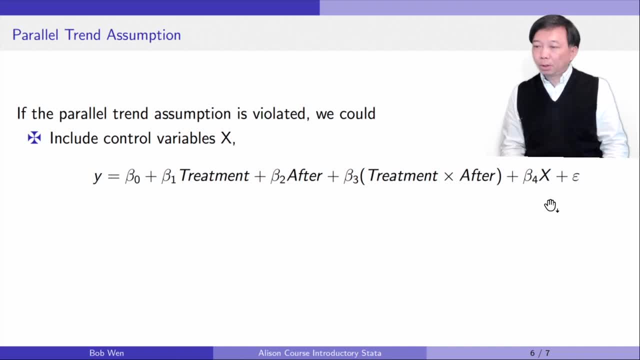 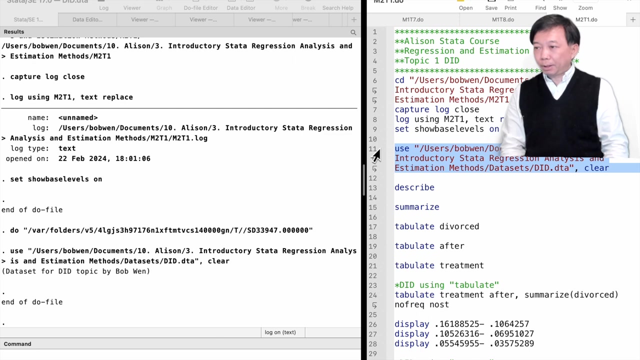 We hope that, after puzzling out the effects of these control variables, the residual outcomes satisfy the parallel trend assumption. As a result, the estimates become more robust and causal. Please download the dataset diddta for this topic. The dataset is about the marital status information. for people living in Illinois and Indiana. The no fault data divorce law took effect in 1973 in Indiana, but it is not implemented in Illinois until 1984.. The no fault divorce law makes divorce less costly. People wonder whether the law increases divorce cases. 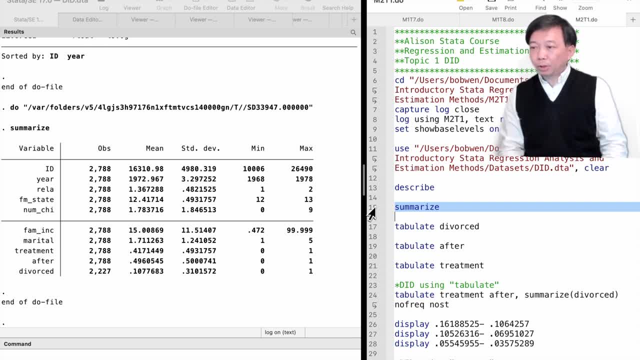 The treatment here is the enforcement of the law in 1973 in Indiana. The treatment group is the families in Indiana, The control group is the families in Illinois. I collected the marital status information before and after the law enforcement for the two states. 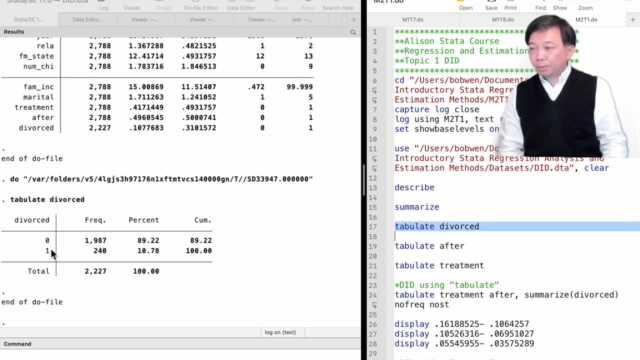 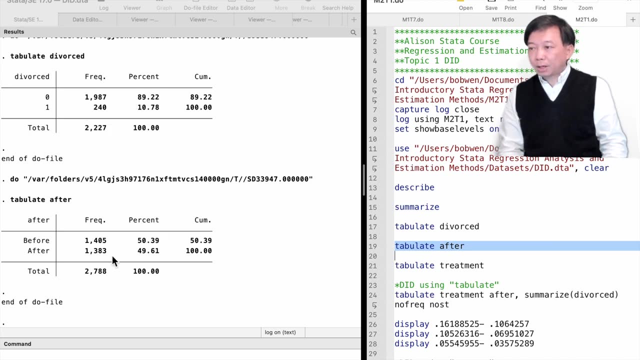 The variable divorced indicates people's marital status. It is equal to 1 if divorced. It is equal to 0 if married. The variable after indicates the time periods after or before the introduction of the no fault divorce law. The treatment variable equals 1 if living in Indiana. 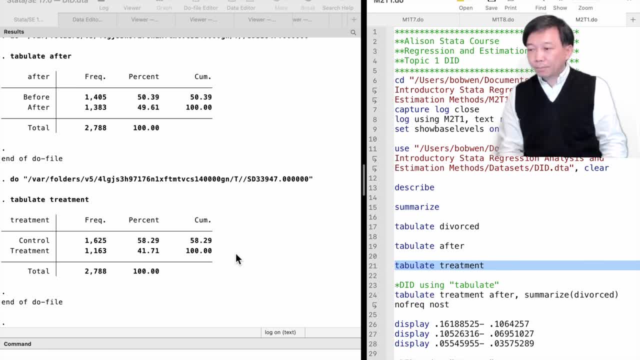 and 0 if living in Illinois. We use the tabulate command to generate a one-way tabulation for the variables and find the percentage of each category. There are various ways to perform a difference-in-differences analysis in Stata. First, we can use the tabulate command to do that. 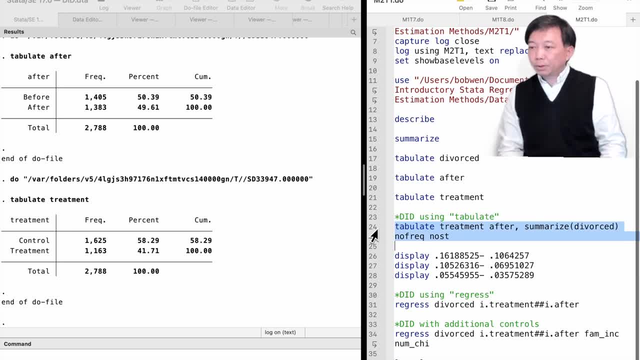 Please refer to the course Introductory Stata Summary Statistics and Data Management for detailed information about the tabulate command. Let's tabulate the statistics in a two-way table. We type tabulate, followed by the treatment variable and the after variable. We use the summarize option. 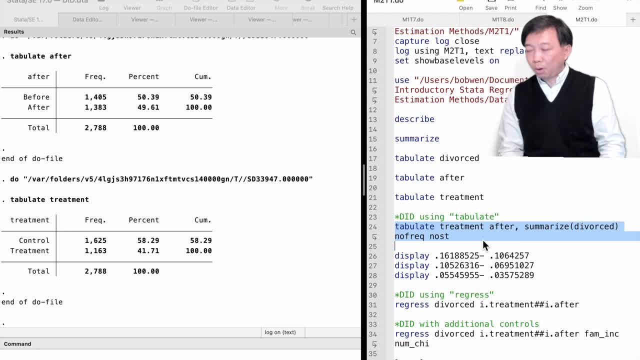 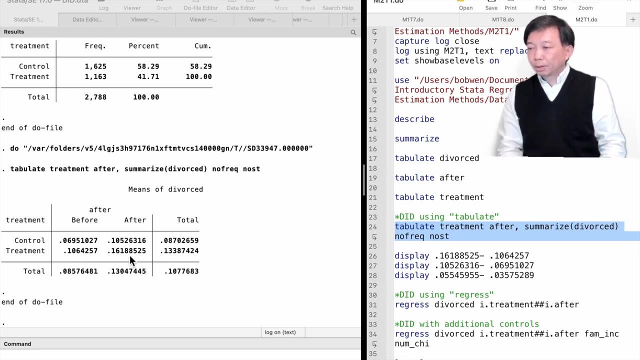 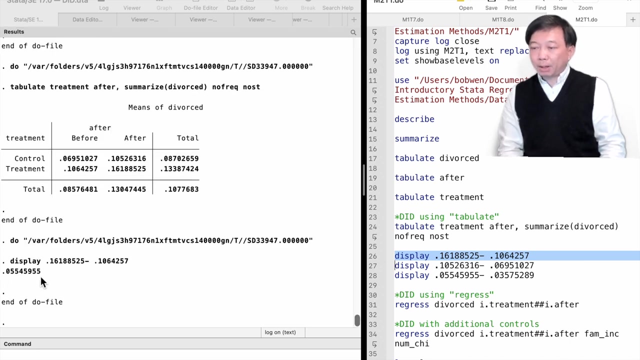 to show the sample mean of the variable divorced. We also apply the no frequency and no standard duration options. Here we have the 2x2 table of the basic difference-in-differences estimates. We see that for the treatment group Indiana the average divorce probability increases by 5.5% points. 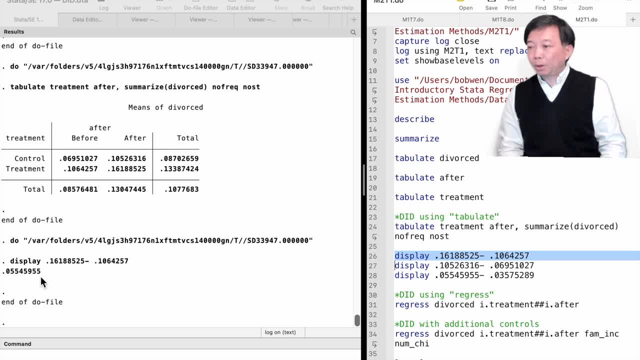 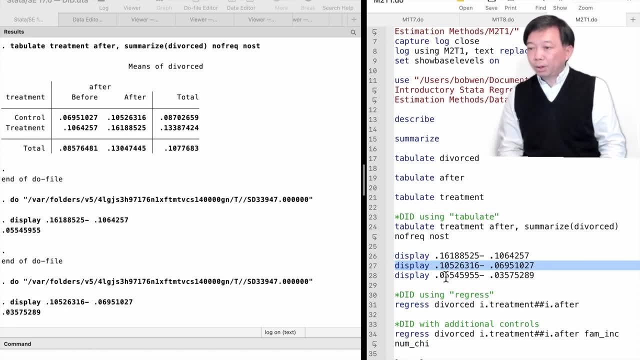 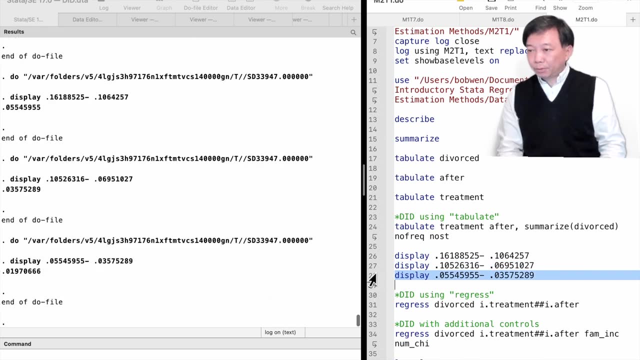 from 10.6 to 16.2.. On the other hand, for the control group Illinois, the divorce probability increases by around 3.6 percentage points. So the difference-in-differences estimate is around 2 percentage points. 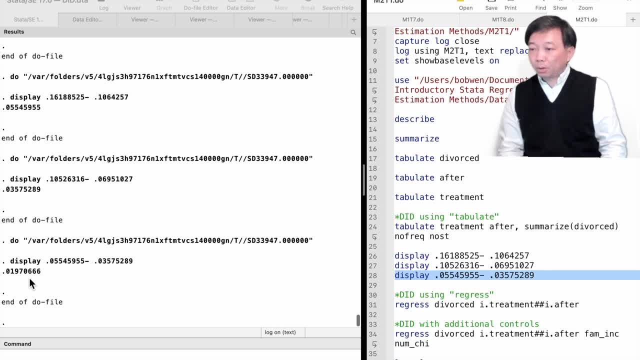 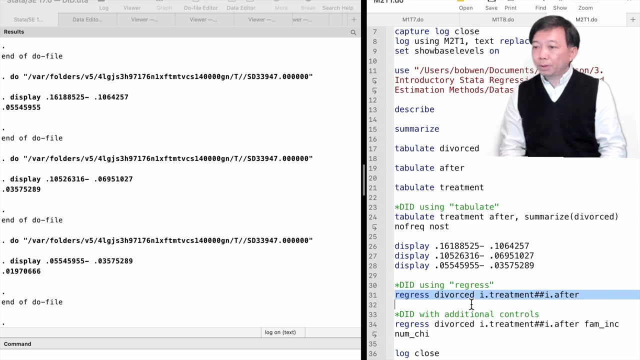 In other words, the no fault divorce law enforced in Indiana actually raises the divorce likelihood by 2 percentage points after we account for the trend of the divorce rate due to reasons other than the law. We can also use the regress command to perform the difference-in-differences regression. 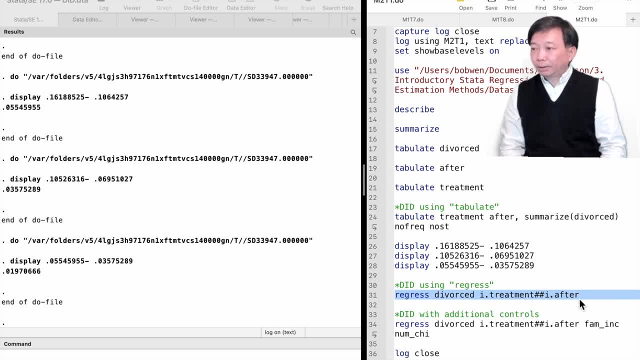 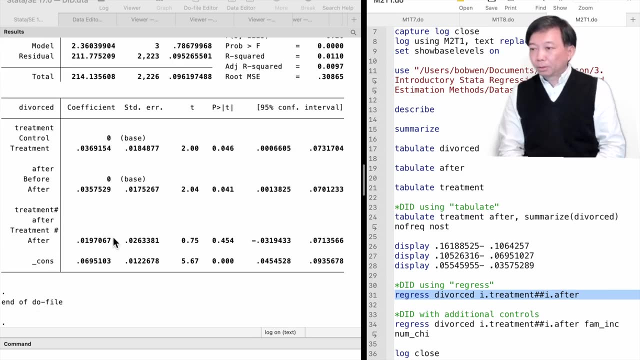 The idoc prefix tells data they are dummy variables. The double hashtags include the interaction term between the two variables, treatment and after in the model. Let's run the regression and here's the output From this table. we know that beta1 is the difference.